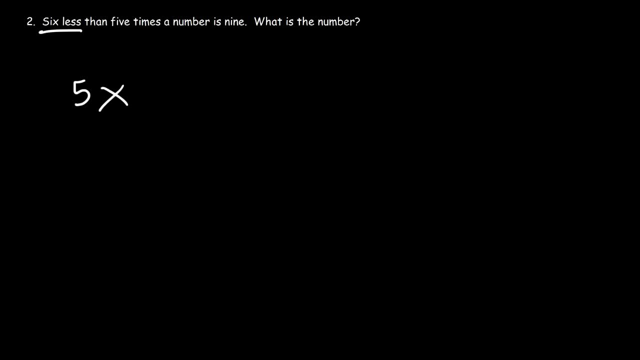 The missing number would represent 5x, And then it's 6, less than 5 times the number, So it's going to be minus 6. Not 6 minus 5x. So be careful when you're dealing with subtraction. You should put: 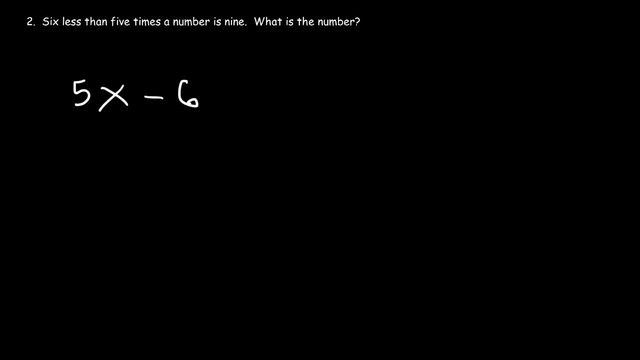 it after, which is usually the way it's going to be. Now we have that word is So we're going to replace with equal. So 6 less than 5 times the number is 9 or is equal to 9.. Now all we need. 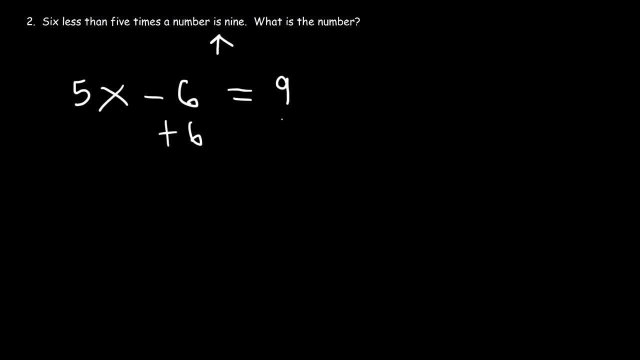 is solve the equation. Let's begin by adding 6 to both sides. 9 plus 6 is 15. And so what we have now is 5x is equal to 15.. Now let's divide by 5.. 15 divided by 5 is 3.. And that is the value of the. 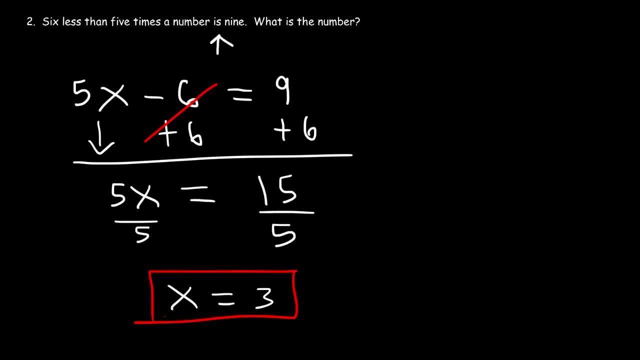 missing number x is equal to 3.. So hopefully you're getting the hang of converting these sentences into equations, And the best way to learn how to do it is with practice. Once you do about 5 or 10 of these problems, you're going to get the hang of it, So just hang in there. Here is another. 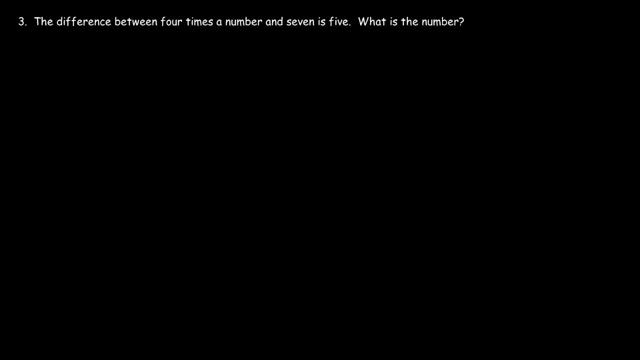 example that we can work on. The difference between 4 times a number and 7 is 5.. What is the number? So let's start with the expression 4 times a number. That's going to be 4x, And then we have 7 and the difference between those two. So we're talking about 4 times. 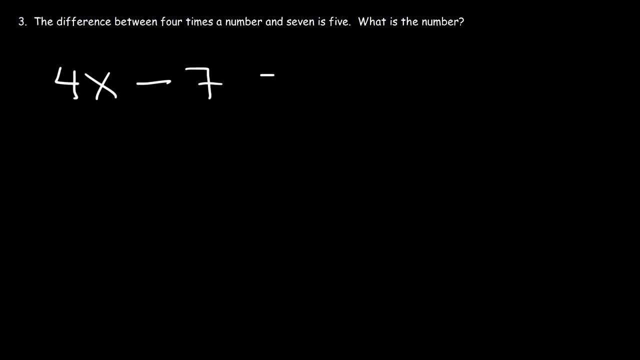 a number. So we're going to have 4 plus 7 is 3, because we're going to have 4 times a number. Yeah, so we get other numbers for all those numbers. Next, we add 4.. We add 7 and 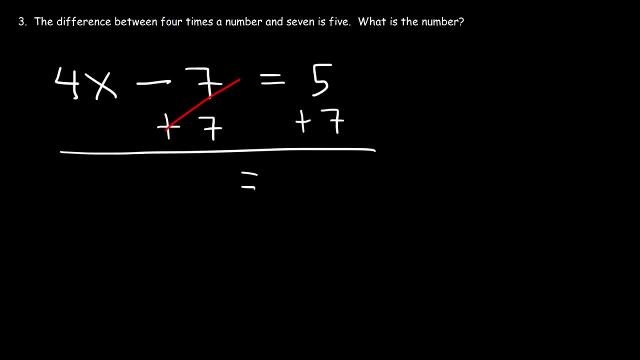 4.. 1 and 1 is 7 and 2 are 2.. So we're going to add 7 to both sides. So we're going to add 7 and 7 to both sides. The passing of number here is 5 and it's 5 plus 7.. So give. 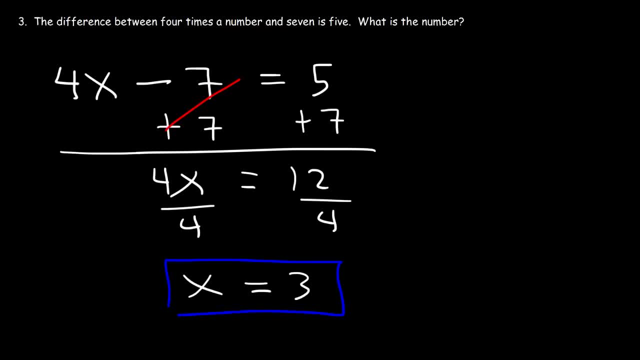 that a probably get Cu n equals double, Cu n equals 2. for this problem. So, whenever you hear the word difference or less than you're dealing with subtraction. If you hear the word some or more than you're dealing with addition. So just keep. 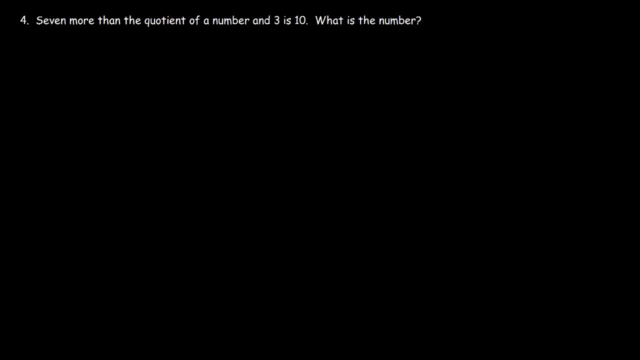 those things in mind. Number four: seven more than the quotient of a number and three is ten. What is the number So seven more? we could simply write seven plus something. Now let's focus on this part: the quotient of a number and three. What does that mean? When you hear the word? 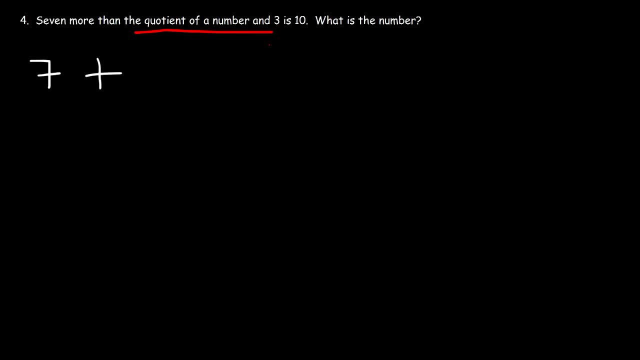 quotient. you need to know that it's associated with division. You need to write some sort of fraction, So you're dividing the number and three, The number. we're going to call it x. You can use n if you want, but I'm just going to use n. 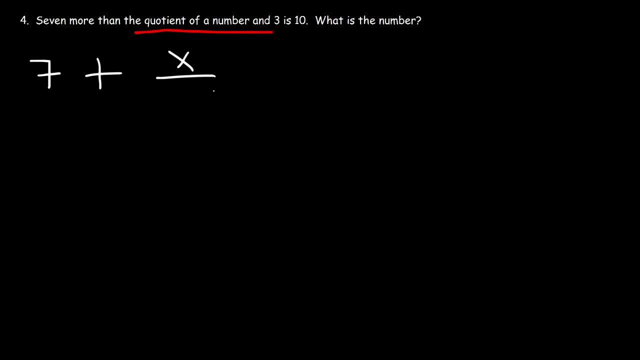 We're going to use x to represent the number that we don't know the value of currently. So the quotient of a number and three is simply x divided by three. That's what it is, And then is or equals ten. So now we can solve the equation. Let's begin by subtracting both sides by seven. 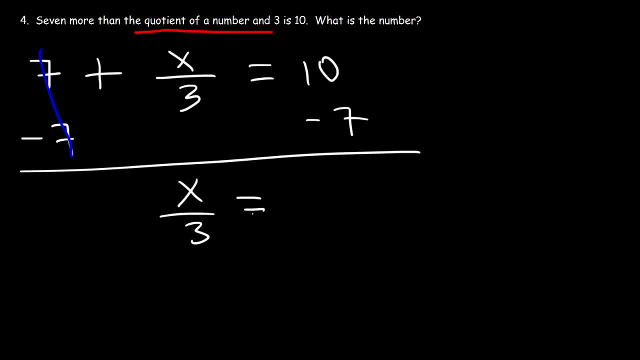 So x divided by three is equal to ten minus seven, which is three. Now let's multiply. Let's multiply both sides by three in order to get rid of the fraction. on the left, Three divided by three is one, And on the right, we have three times three, which is nine. So that is the number. 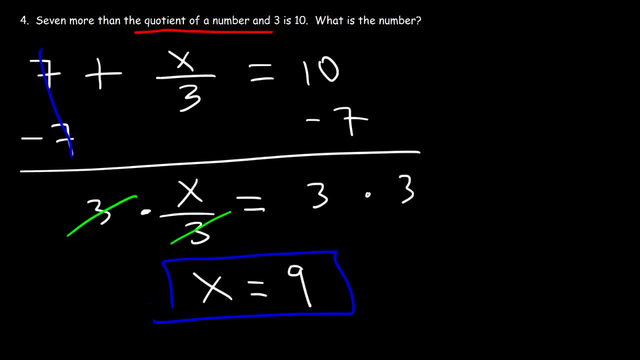 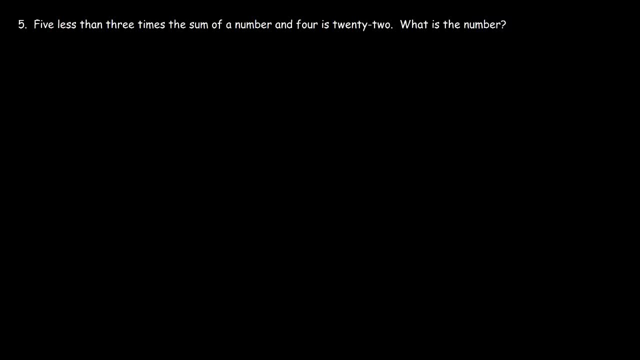 X is nine. Number five, Five less than three times the sum of a number and four is 22.. What is the number? So how should we begin? Let's focus on the sum of a number and four, So the sum represents addition. 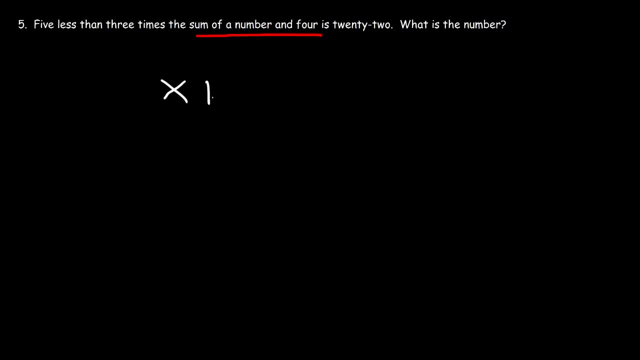 So x plus four. x is the number, That's the sum of the number and four. And then we have the expression three times the sum of a number and four. So this is going to be three times X plus four. So we are. So we are going to put the three outside and 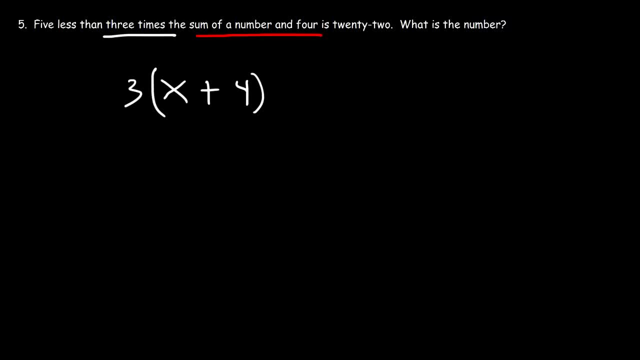 enclosed the x plus four within parentheses, And then we have expression five less than all of that. So we could put the minus 5 and all of this is, or equals 22.. So this is the equation that we now have. Let's go ahead and solve it Now. let's begin by distributing the 3.. 3 times x is 3x and 3 times 4. 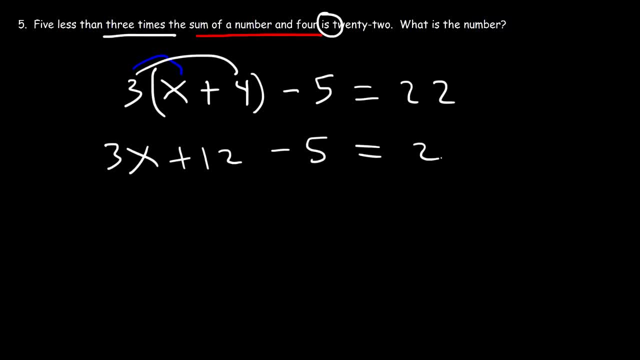 is 12.. Next let's combine like terms. On the left side we can combine 12 and negative 5.. 12 minus 5 is positive 7.. Now let's subtract both sides by 7.. 22 minus 7 is 15, and if we divide both sides by, 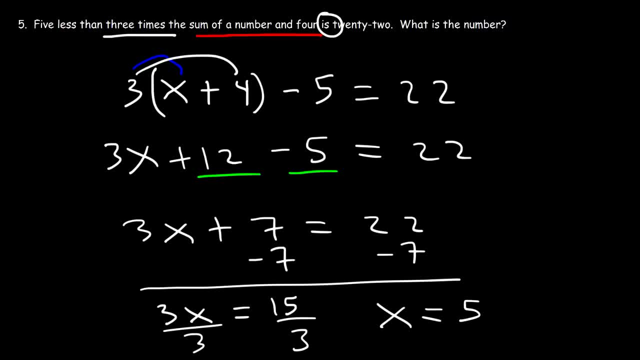 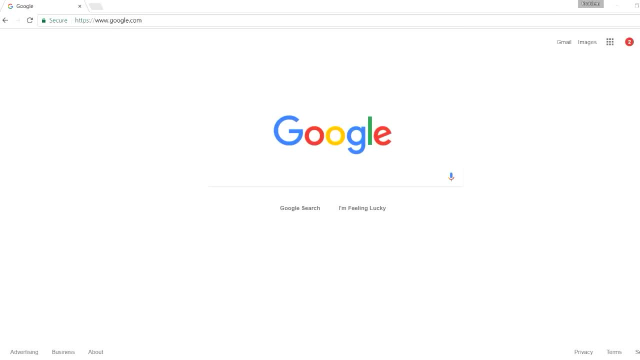 3, 15 divided by 3 is 5., And so that is the value of the missing number. x is equal to 5.. Now I want to show you one of my algebra courses that might be useful to you if you ever need it. 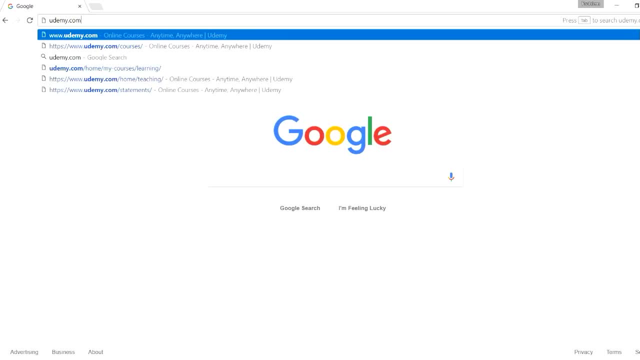 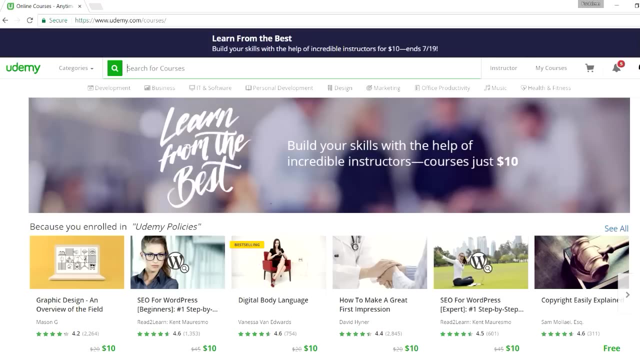 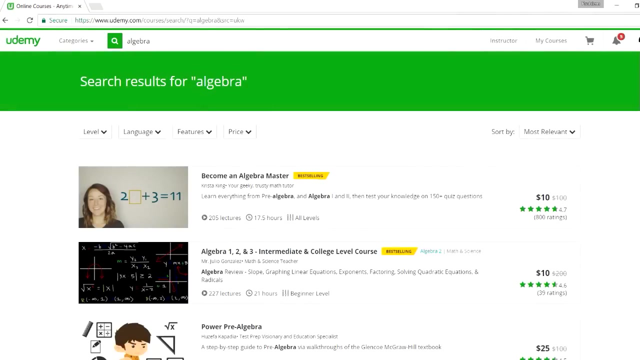 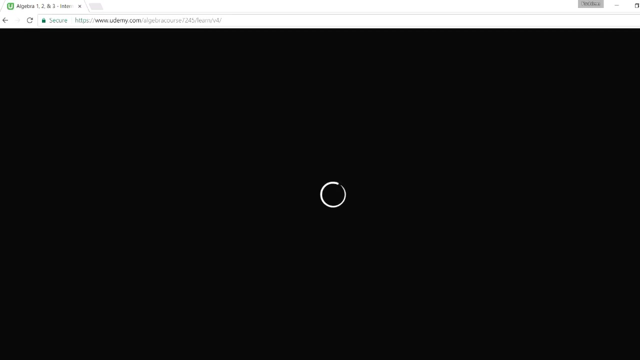 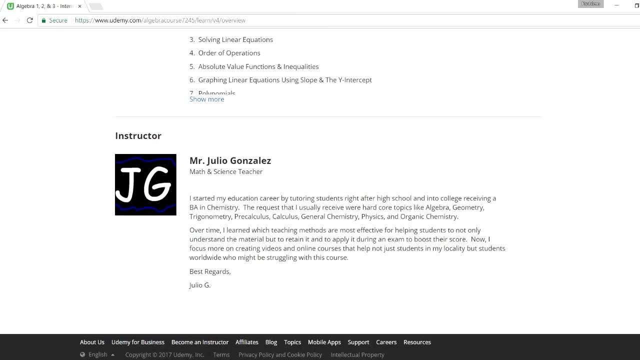 So go to udemycom Now. in the search box just type in algebra and it should come up. So it's the one with the image with the black background. So if you select that option and if you decide to go to course code, you can go to course code. So if you go to course code, you can go to course code. 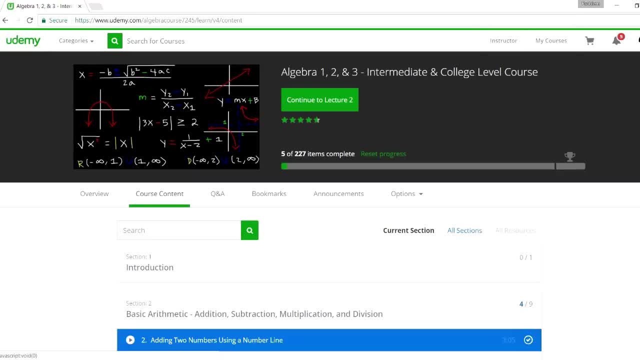 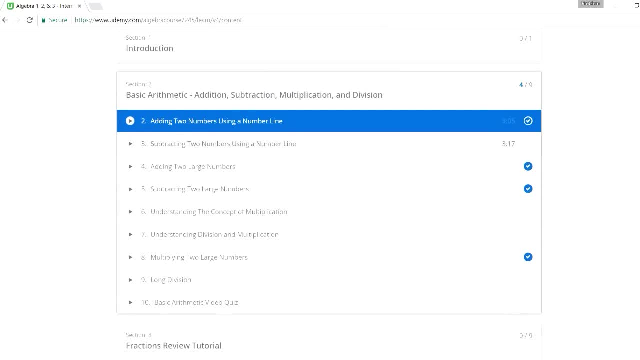 content. You can see what's in this particular course. So the first section, basic arithmetic- for those of you who want to focus on addition, subtraction, multiplication and division, And it has a video quiz at the end. It's a multiple choice video quiz. You can pause it. 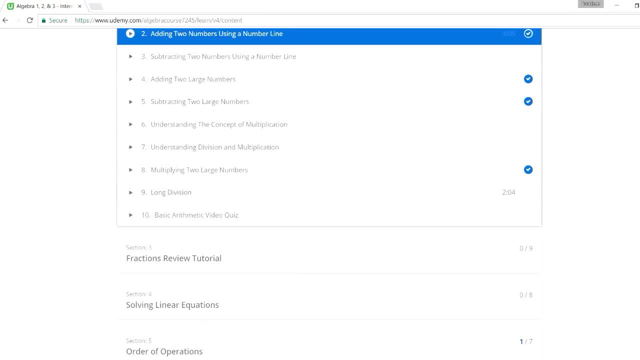 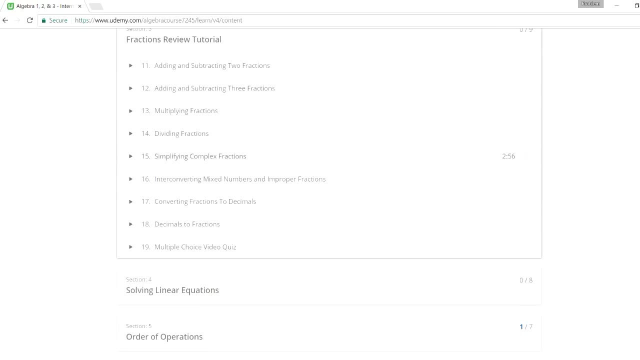 work on the problems and see the solutions. It covers long division, multiplying two large numbers and things like that. The next tutorial is on fractions: Add in, subtracting fractions, multiplying, dividing, Adding fractions, converting fractions into decimals and so forth, So you can also take a look at that. 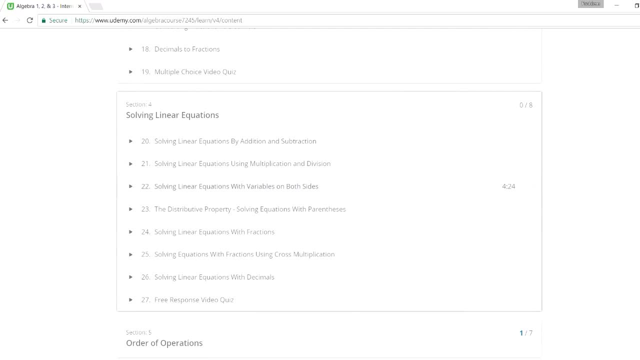 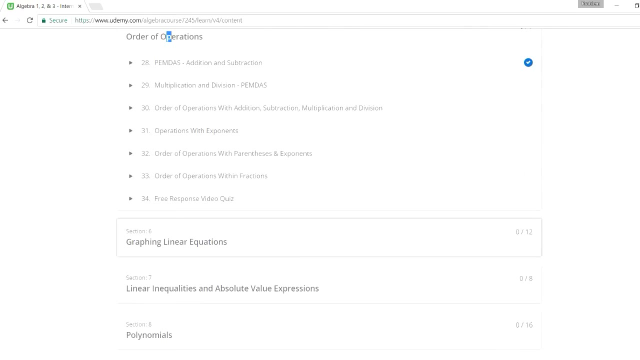 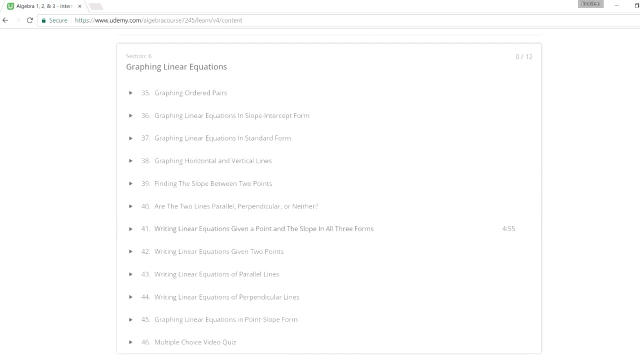 Next, solving linear equations, which we covered, And just more examples if you need more help with that. The next topic, order of operations, which is also useful: Graphing linear equations. You need to know how to calculate the slope. You need to be familiar with the slope intercept form standard. 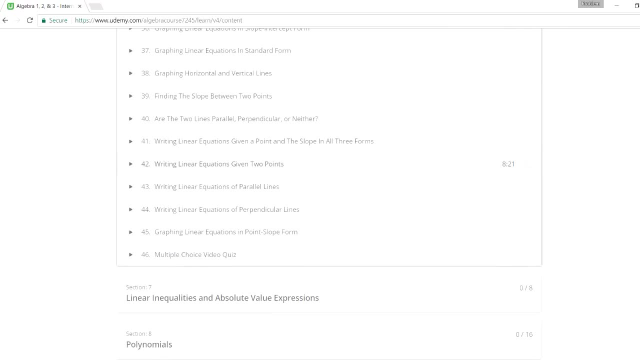 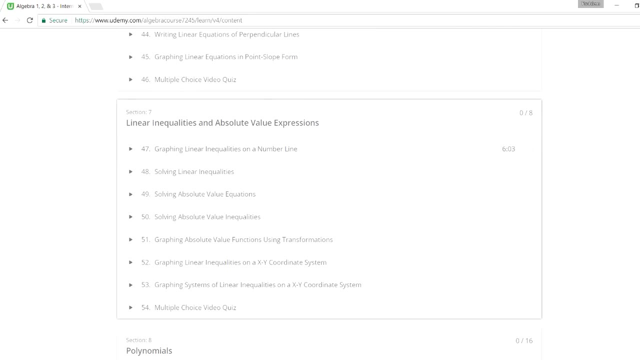 form and just how to tell if lines are parallel. So if you're familiar with the slope, intercept, form, parallel, perpendicular and so forth, And it's a quiz that goes with that as well. The next topic is on inequalities and absolute value expressions, which are also seen in a typical 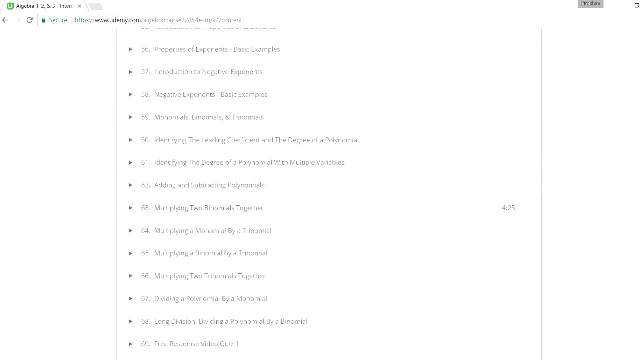 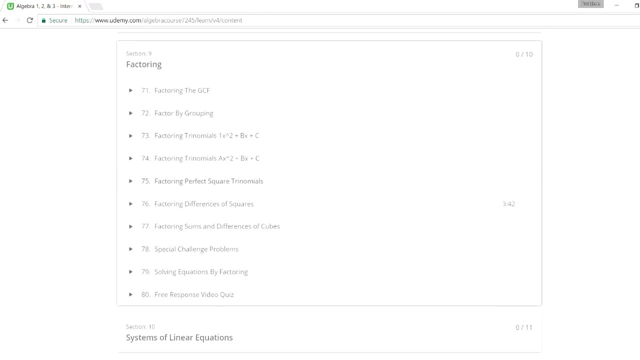 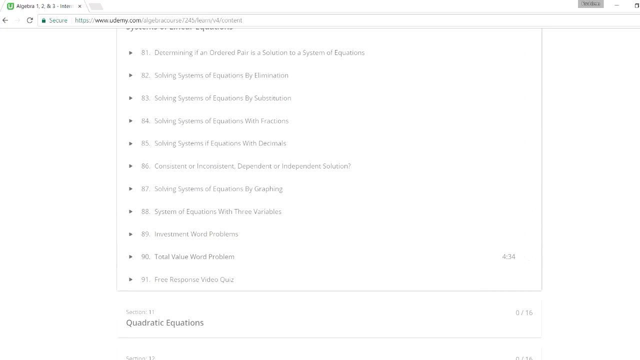 algebra course, And then we have polynomials And that's a long section, And then factoring You- just that's another topic you need to master. And then system of equations: You can solve it by elimination, substitution. There's also word problems as well. 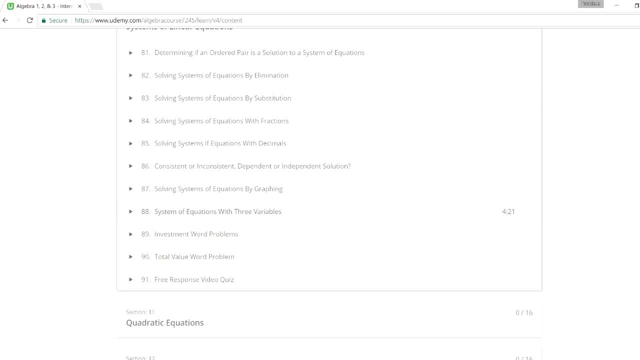 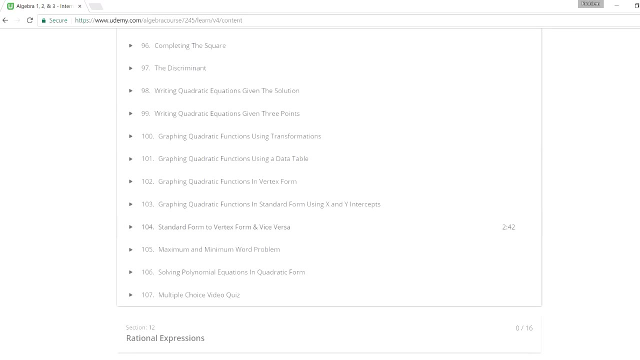 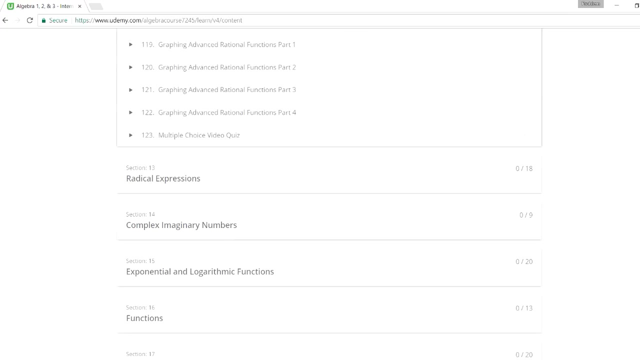 Sometimes you got to solve equations with three variables- x, y and z, So that could be helpful. Next, quadratic equations: How to use a quadratic formula, How to graph them, How to convert between standard and vertex form. And then you have rational expressions And radical expressions. 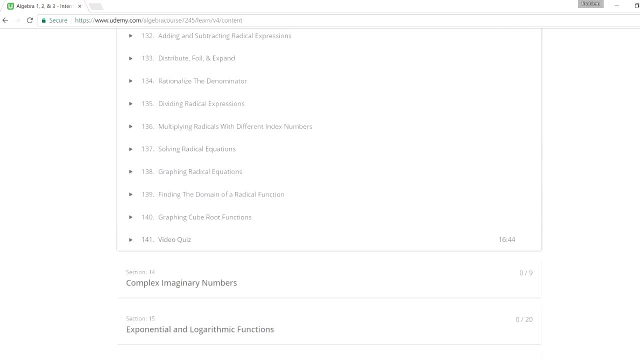 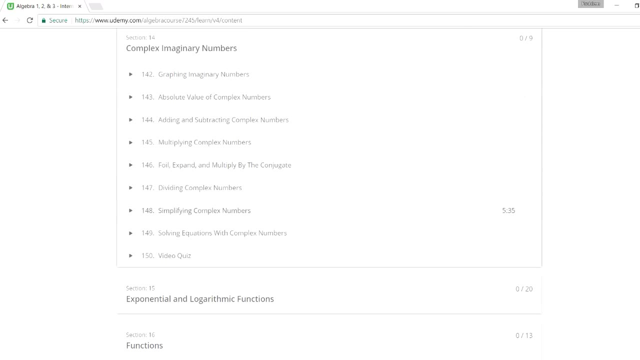 Solving radical equations, Simplifying it, Things like that. And every section has a quiz So you can always review what you've learned if you have a test the next day. So here we have complex imaginary numbers. You need to know how to simplify those Exponential functions, Logs. 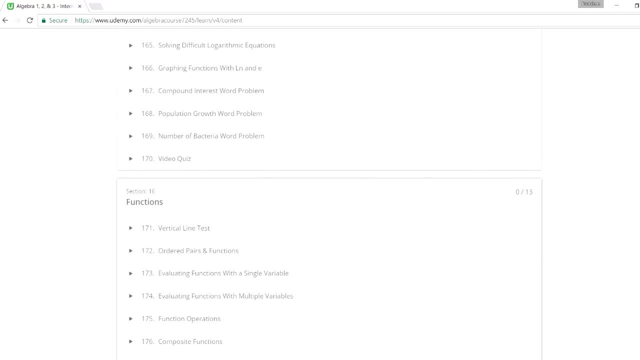 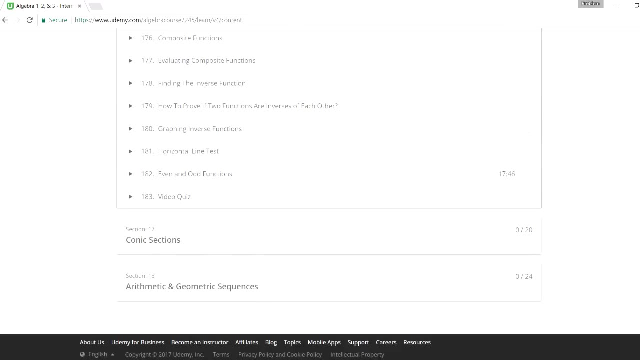 I have a lot of videos on logs, And then this is just functions in general: Vertical line tests, Horizontal line tests, How to tell if a function is even or odd, And then conic sections, Graphing circles, hyperbolas, ellipses, parabolas and things like that. There's two video quizzes. 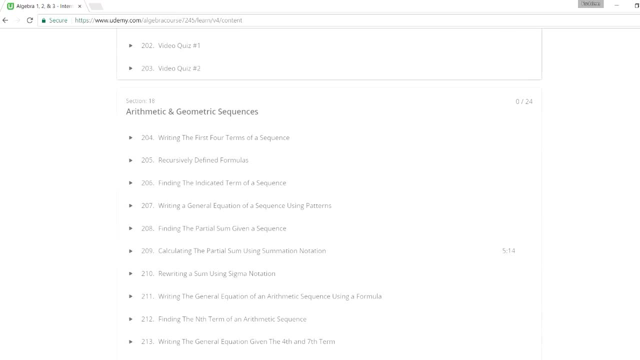 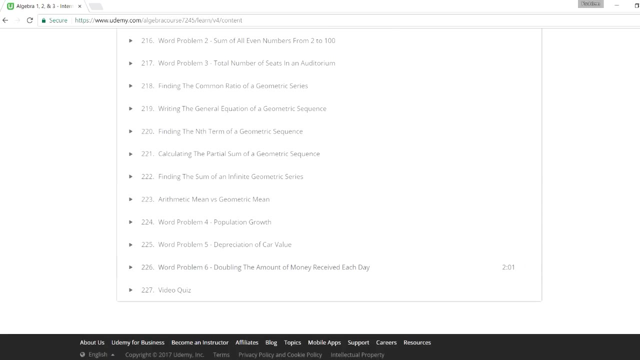 because it's actually a long section, And finally arithmetic and geometric sequences. So that's my algebra course. if you want to take a look at it And let me know what you think. 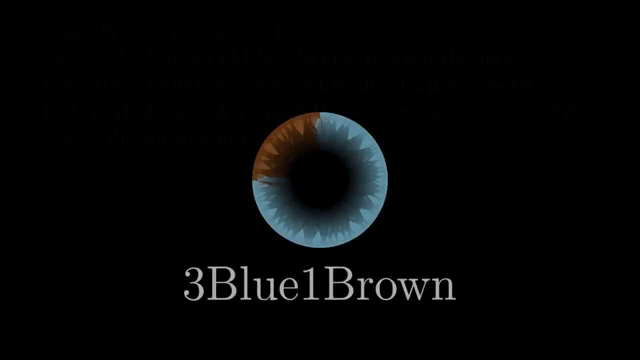 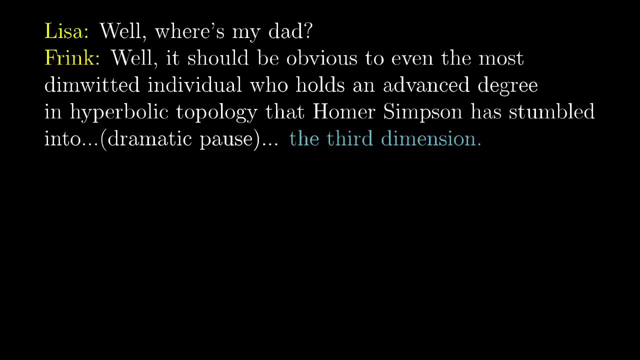 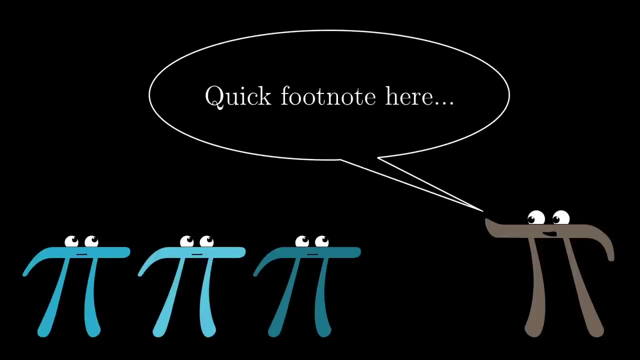 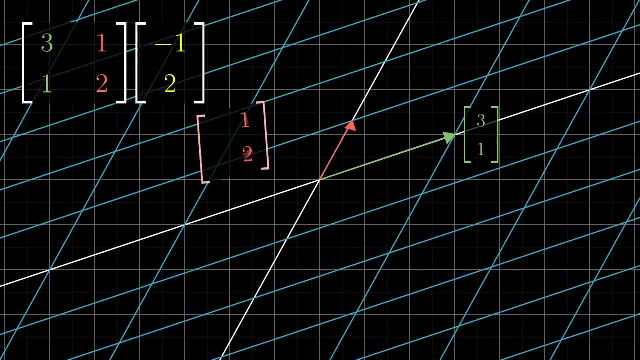 Hey folks, I've got a relatively quick video for you today, just sort of a footnote between chapters. In the last two videos I talked about linear transformations and matrices, but I only showed the specific case of transformations that take two-dimensional vectors to other. 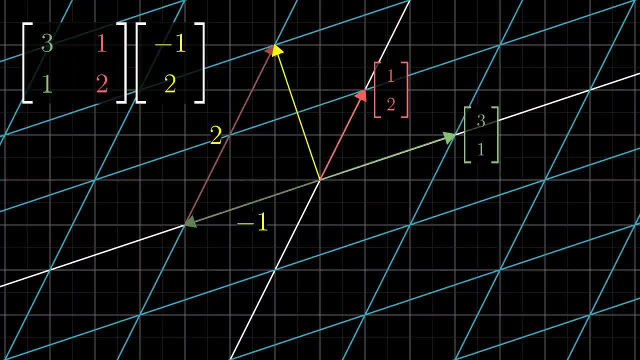 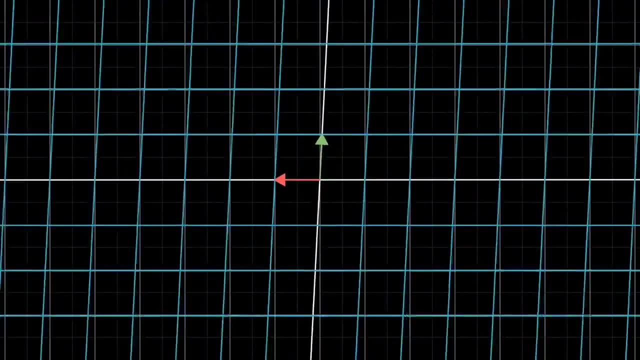 two-dimensional vectors In general. throughout this series we'll work mainly in two dimensions, mostly because it's easier to actually see on the screen and wrap your mind around. But more importantly than that, once you get all the core ideas in two dimensions, they carry.